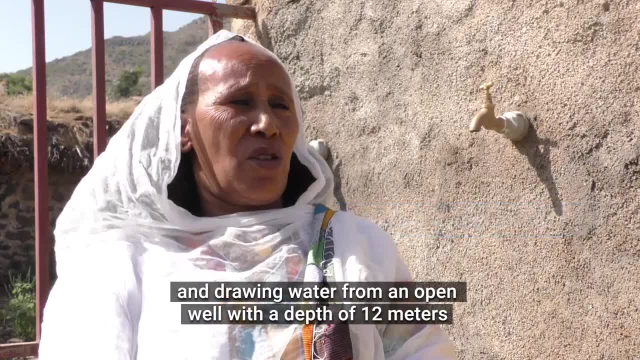 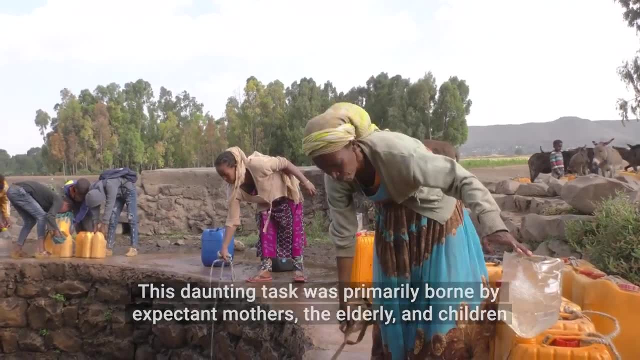 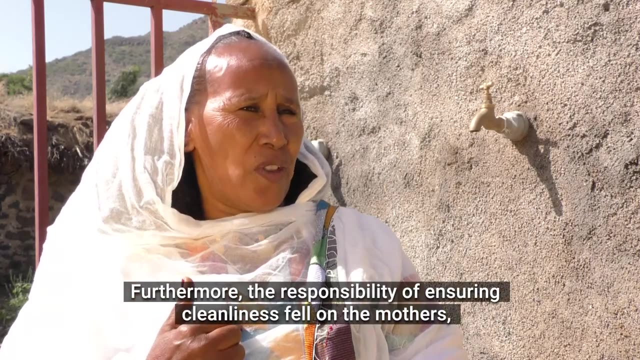 If the water did show surface water in the water, other people would have to search for it. The water would be 해석ع. When water flows from the well, water will drop closer to the wall, but later, as the river moves, it will throw away the water that has fallen in the water. 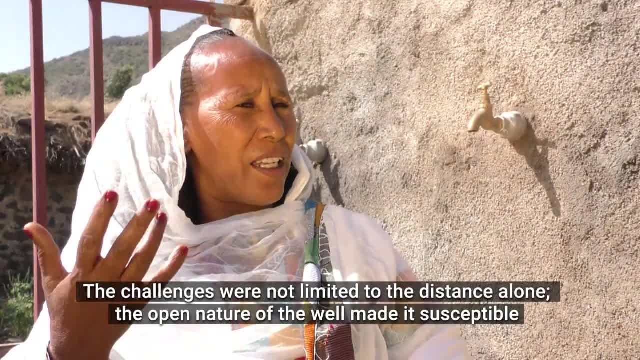 As a matter of fact, the water is filled up with water in a way that it can only be filled with water by means of water, Because when water flows from the well, water can be gushed out from the well. The water will flow from the well, but not from the well. 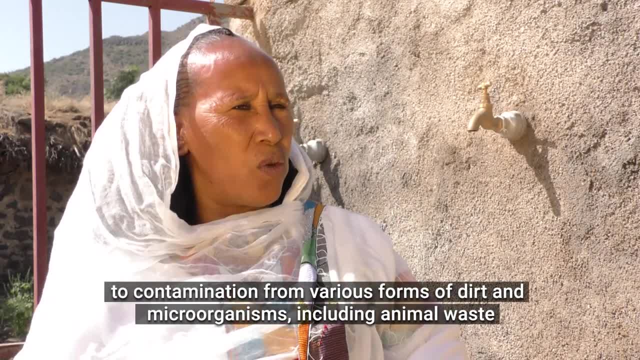 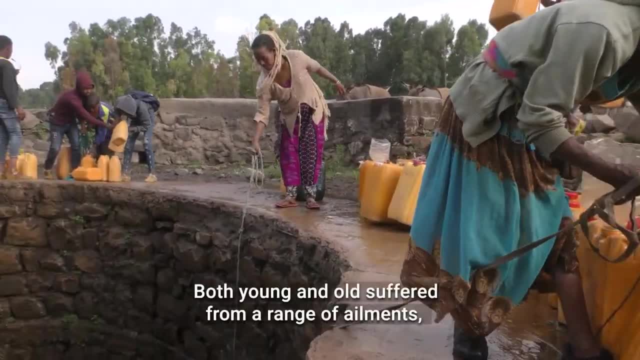 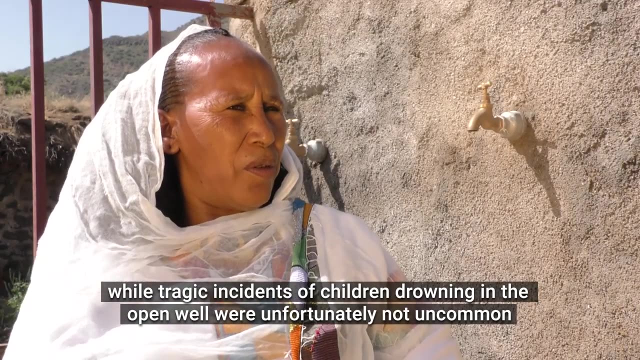 That's it. We had to find a way to take them to the hospital. The doctors said the woman is lying in the hospital. The doctor said he is sick. We have to go to get help to take him. We have to go to the hospital. 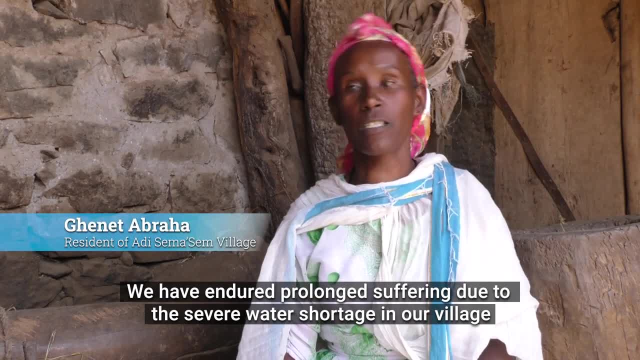 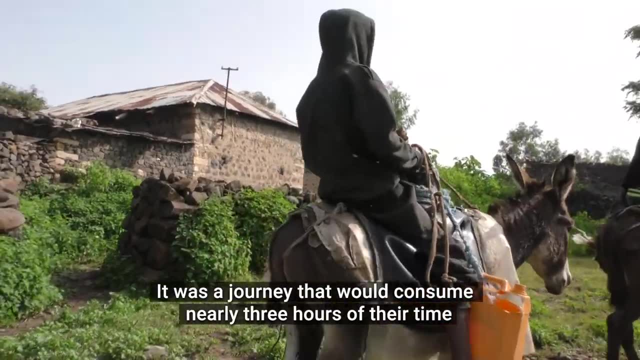 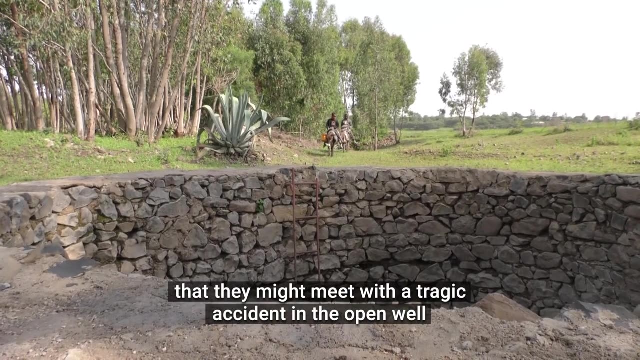 My husband was a doctor. We went and took him to the hospital and we have been working for three years. We have been working for hours, We are working with the government, but we are not doing anything. We are only running to get our food supplies. 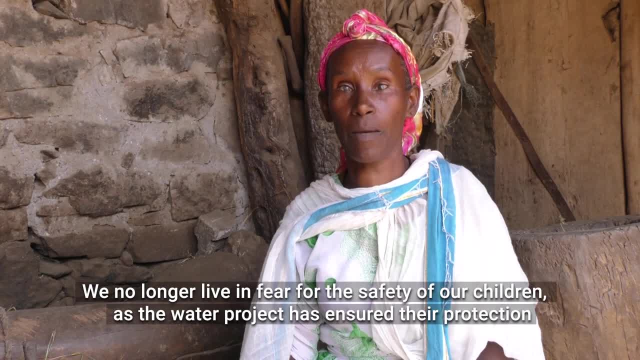 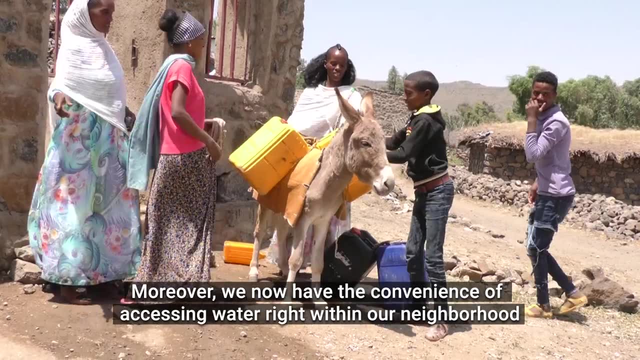 We are not going to sell anything to the government. We are just running to get our food supplies. We can't do anything, but we will do our best. The government is working for us, but we don't have any food to sell. 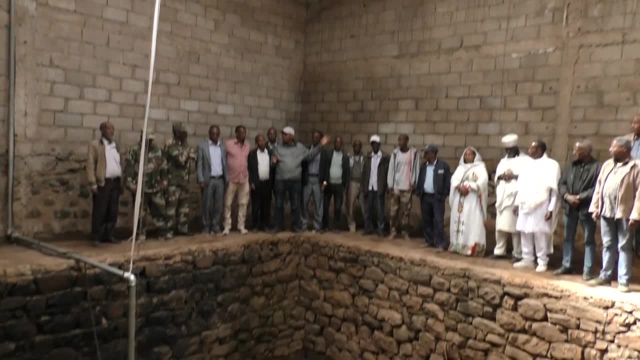 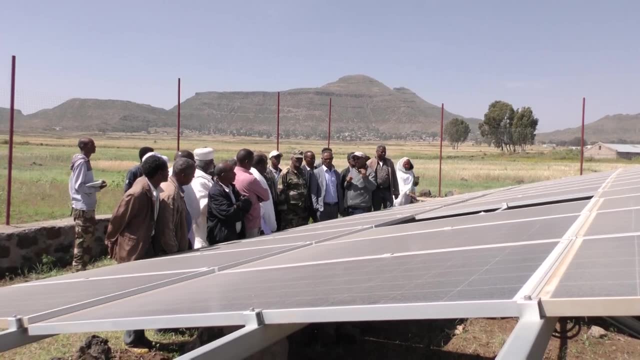 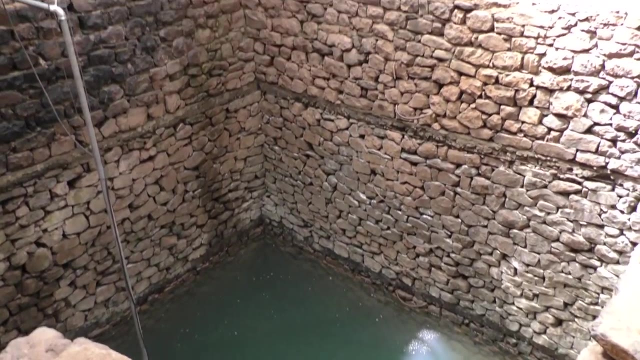 Recognizing the urgent need for a reliable and clean water supply, the government of the state of Eritrea collaborated with development partners to address this critical issue, which has resulted in the successful installation of a solar-powered water project in Addis Amasem village. 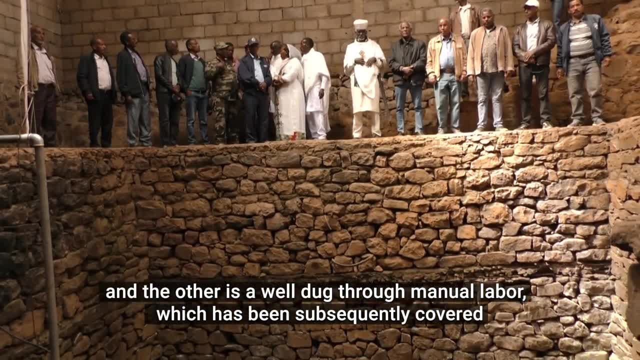 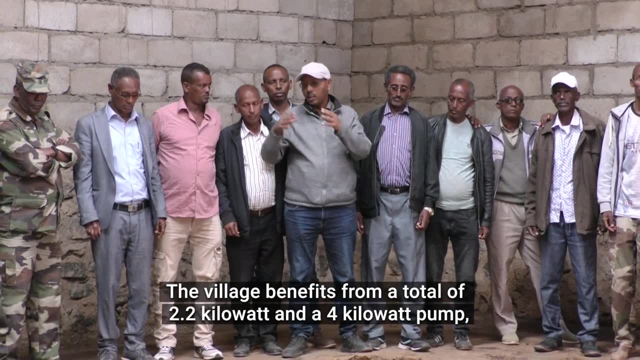 The water supply was disposed by the government of Addis Amasem and was regulated by the government of the state of Addis Amasem. The power of the water pump, which is about 140 kilowatts, was delivered to the village via a five-meter-high waterway. 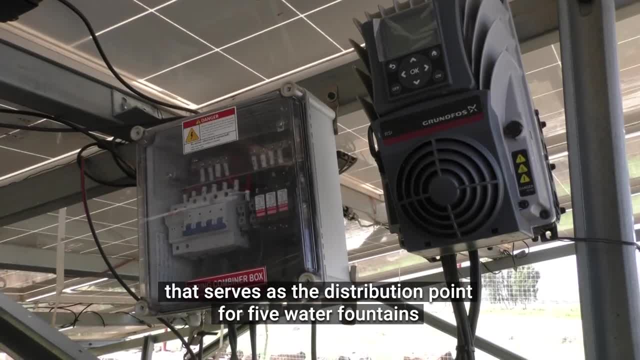 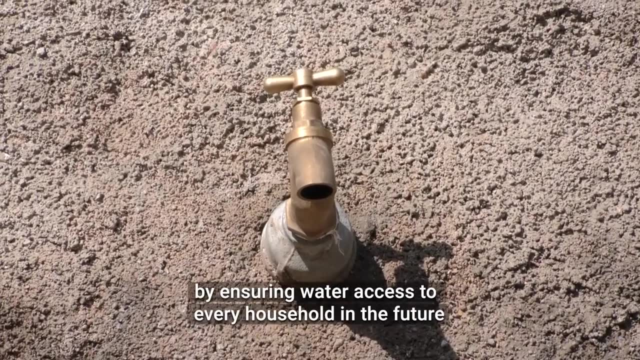 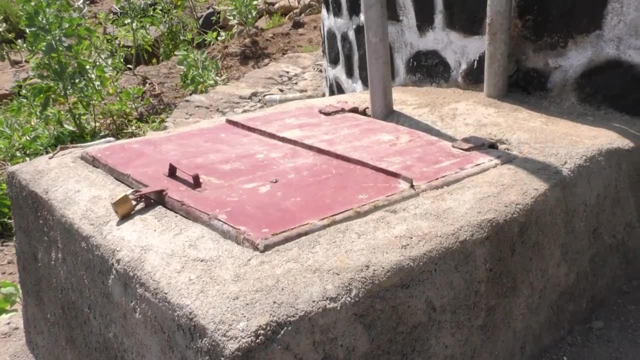 The five-meter-high waterway is a good example of the development of the Eritrean people. The Eritrean people were very happy with our new waterway. This is where we are with our efforts. The project, comprising five installations, brought the source of water closer to the 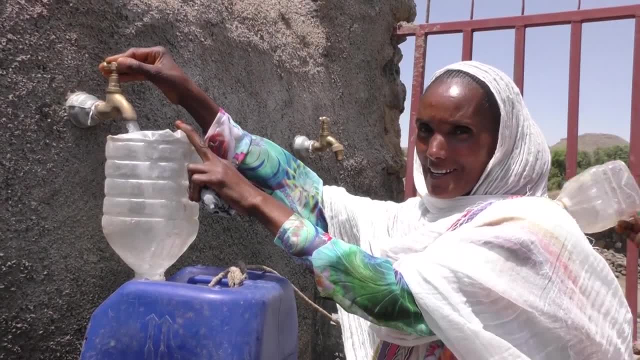 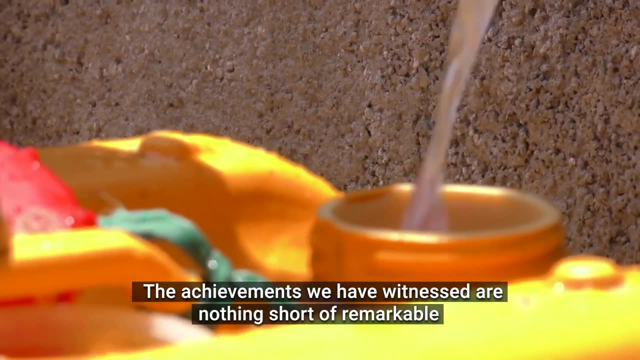 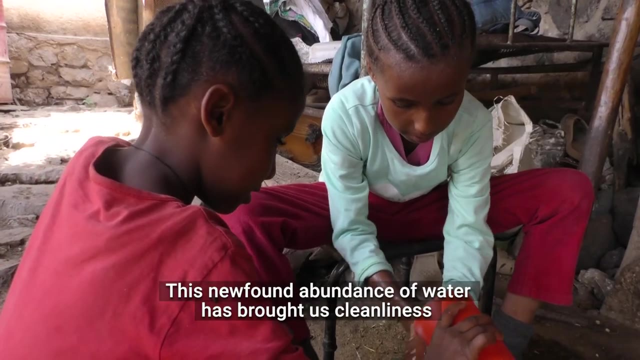 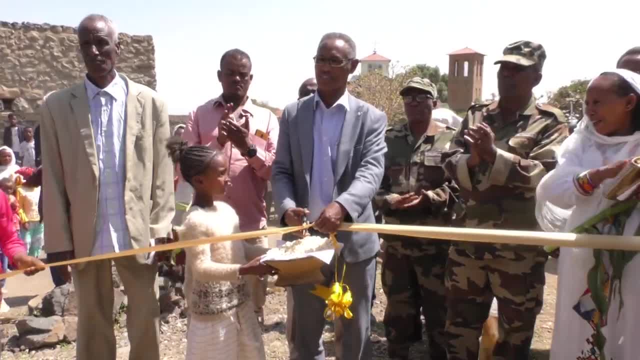 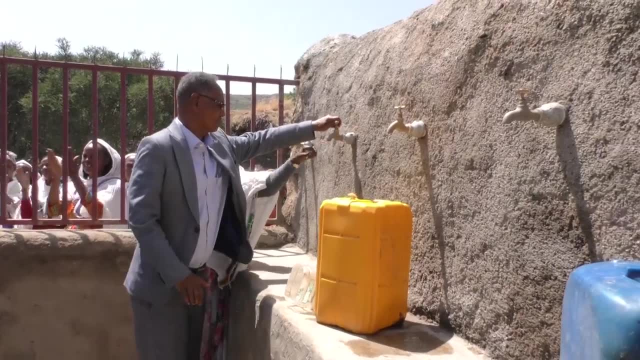 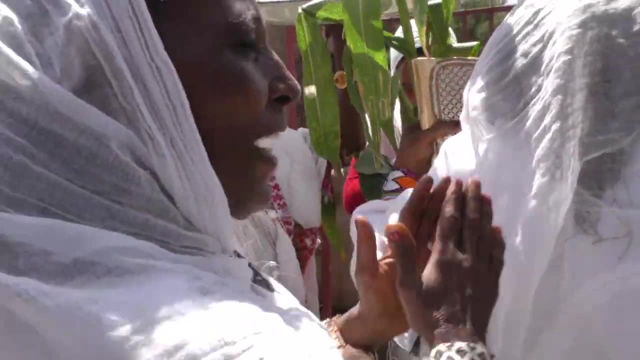 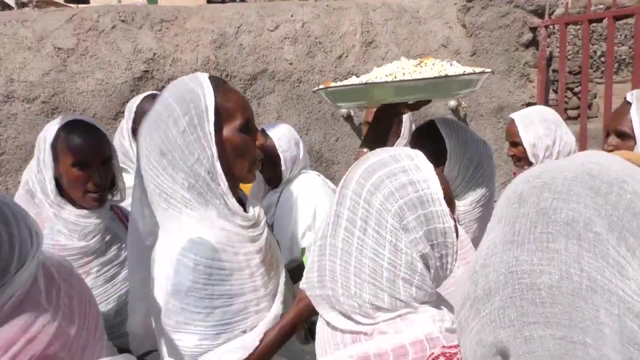 we have never forgot this, because it was like a museum. The inauguration of one of these installments was celebrated by the community on September 30, 2023, marking a significant milestone in their journey towards a better quality of life. The impact of the solar-powered water project on the lives of the residents of Adissam-Assem. 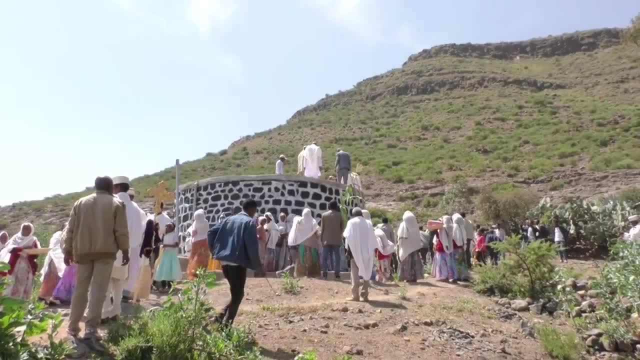 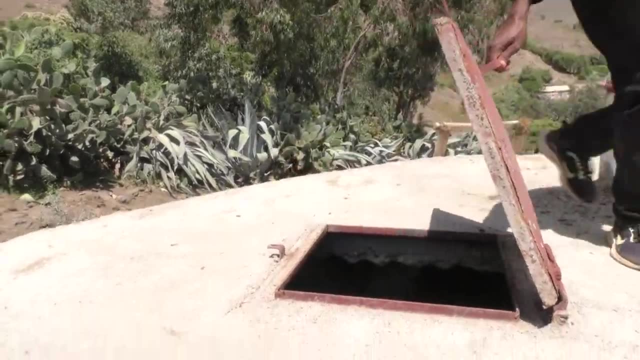 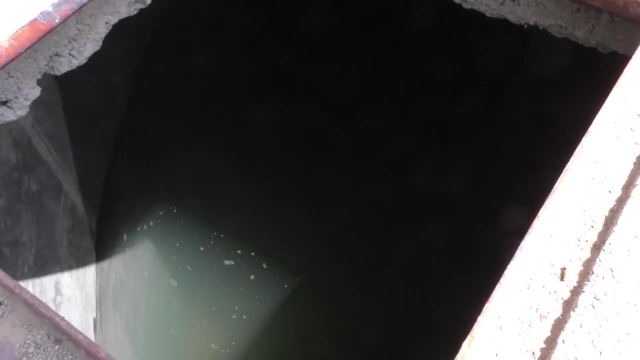 cannot be overstated. The project has brought about a remarkable transformation ât in their everyday lives. No longer burdened with the physical strain and health risks associated with fetching water from distant and contaminated sources, the villagers now have access to clean and safe water. 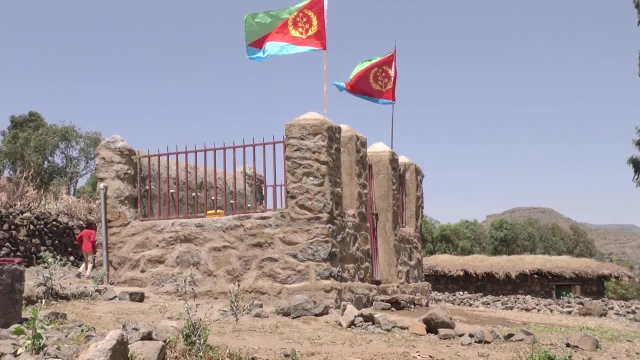 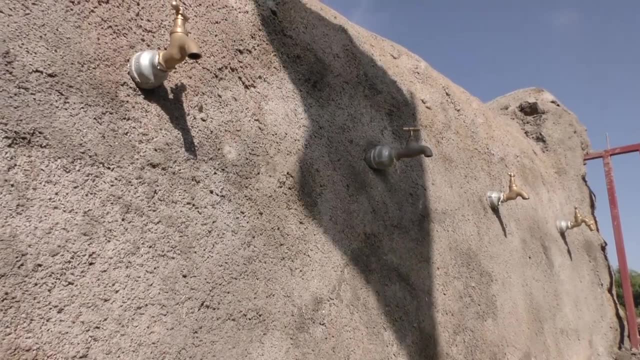 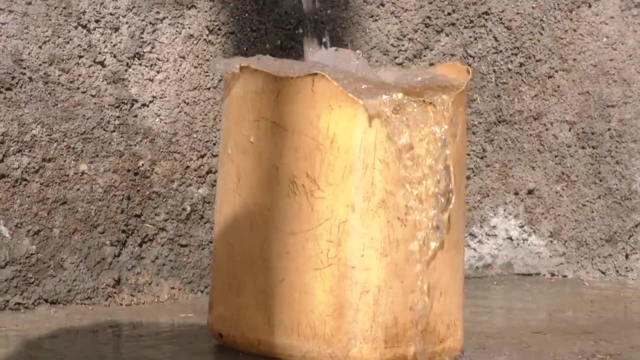 within their immediate vicinity. This newfound accessibility has not only improved their overall health and well-being, but has also alleviated the burden of water collection, allowing community members, particularly women and children, to invest their time more productively in education, livelihoods and community development. 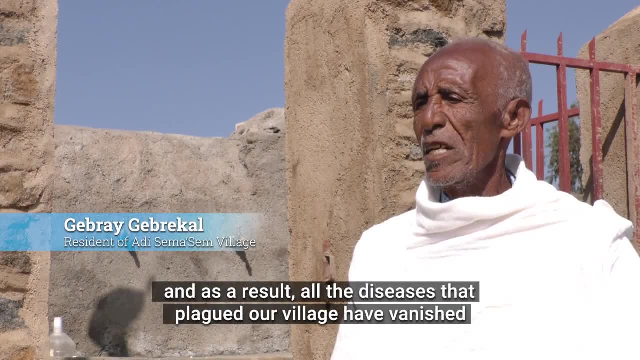 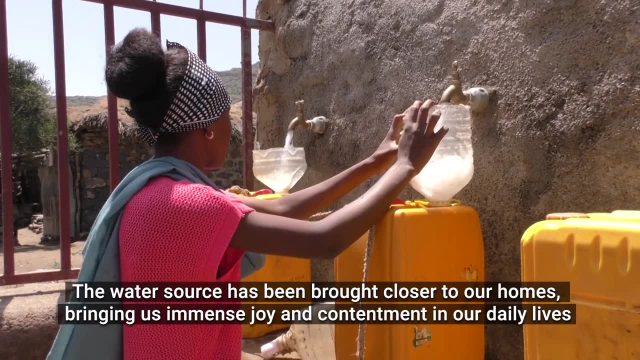 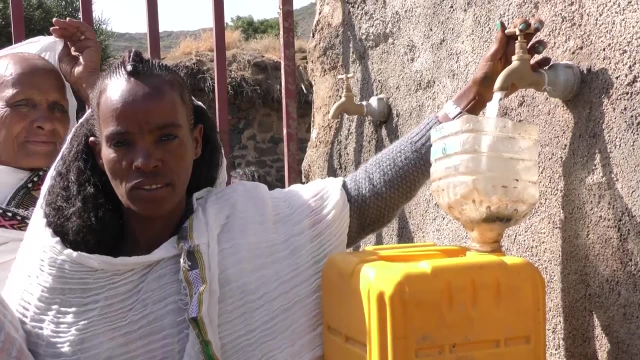 The water that we use to water our fields is the only source of water for us. The water that we use to water our fields is the only source of water for us. The Addis-Am-Assam Solar Powered Water Project stands as a testament to the positive 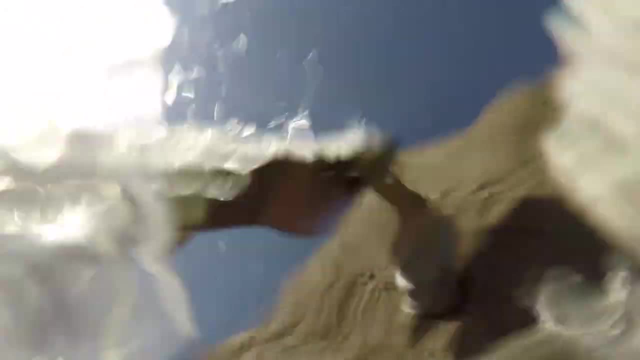 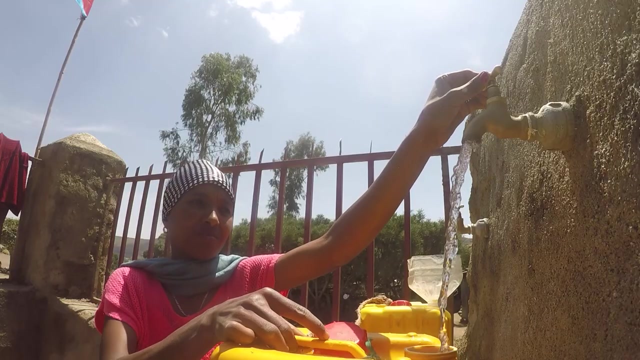 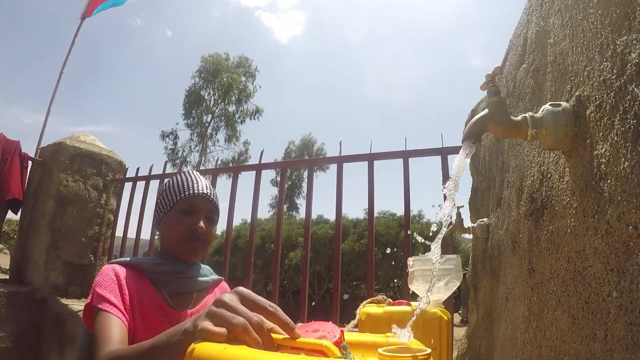 outcomes that can be achieved through effective collaboration between the government and development partners. By bringing clean water closer to home, this project has significantly improved the lives of over 1,000 residents, eradicating the risk of waterborne diseases and alleviating the physical strain associated with fetching water. 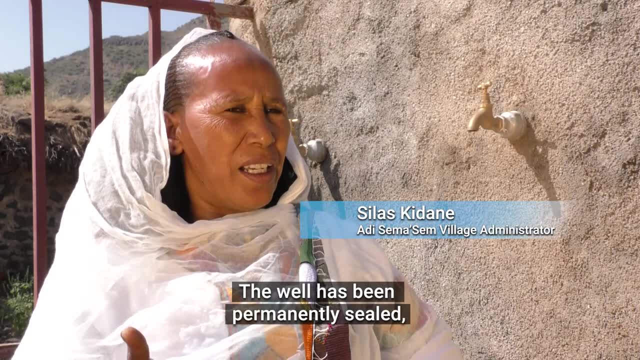 from distant sources. The water that we use to water our fields is the only source of water for us. The water that we use to water our fields is the only source of water for us. The water that we use to water our fields is the only source of water for us.